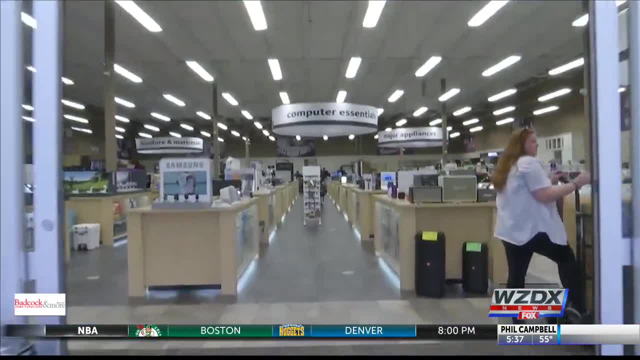 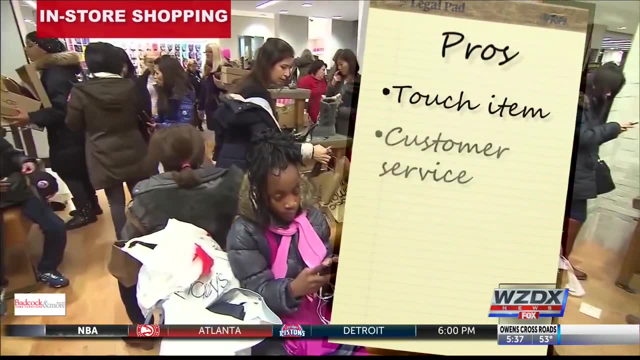 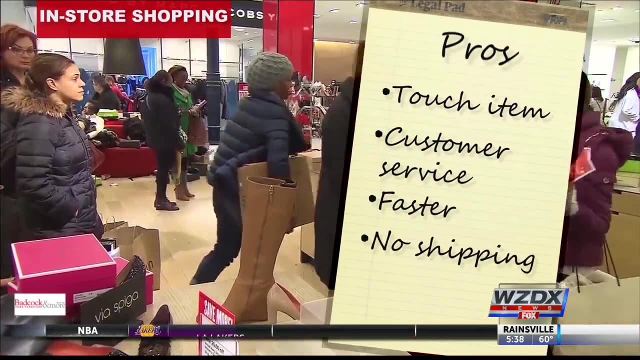 But if actually setting foot in an establishment is your MO, some pluses. You actually get to interact with an item before you drop some change and customer service is a whole lot easier. It's instant gratification. We know you're impatient. No shipping costs, nor return costs because you're the shipper And looking to kill some time on a Saturday, A shopping trip sounds like a plan. 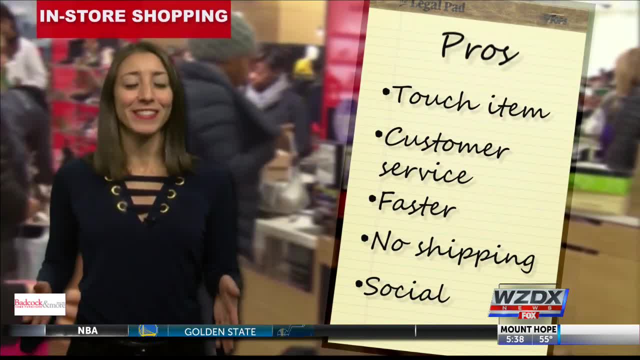 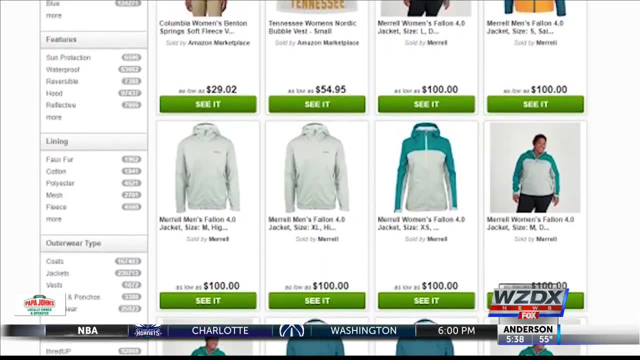 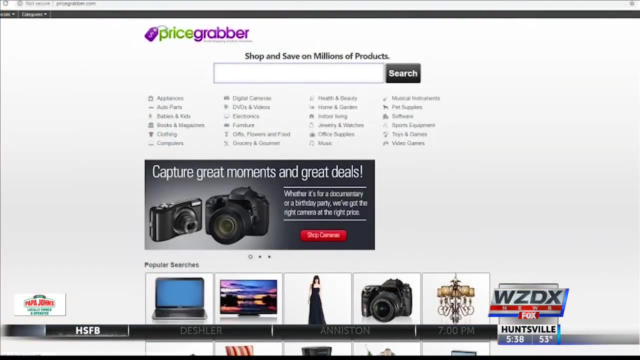 So right now you might be saying: duh, Renata, we know this, Stay with me here. we're going through it because it'll come in handy later. Keep in mind: online price comparison can be way easier than driving around to 15 different stores. There are Smart Shopper apps and sites for this. like on Price Grabber, You can compare apps to your favorite store. 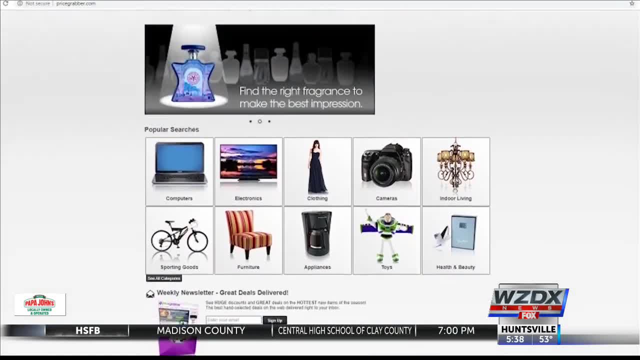 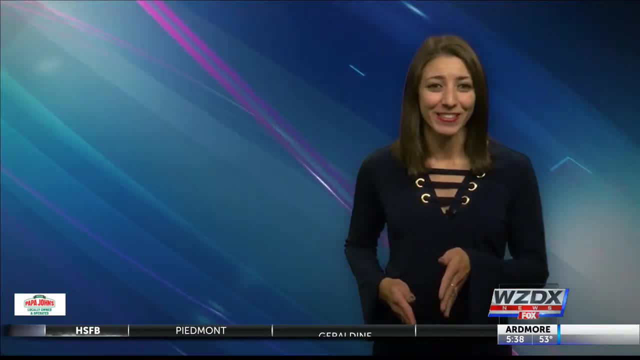 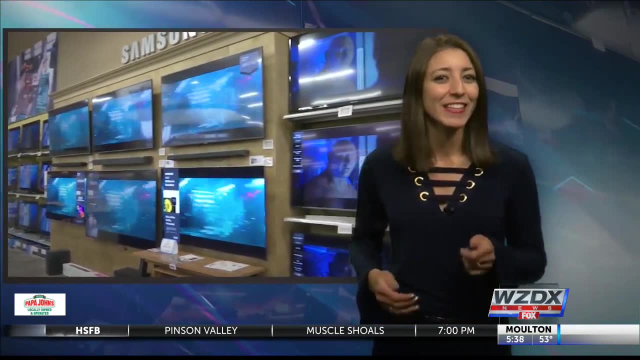 You can buy everything, Then, if you still want, go to the store. Don't forget about shipping costs. Also, look for discount codes online. Alright, so what if you're shopping for something specific Like a TV? Bringing in the data on this? one tech advice website, LifeWire, went through our trusty list and here's their final verdict on prices. 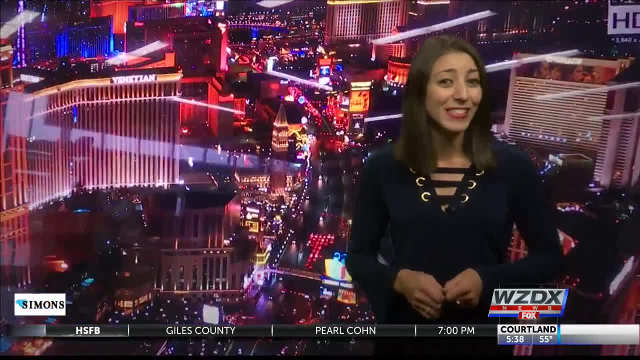 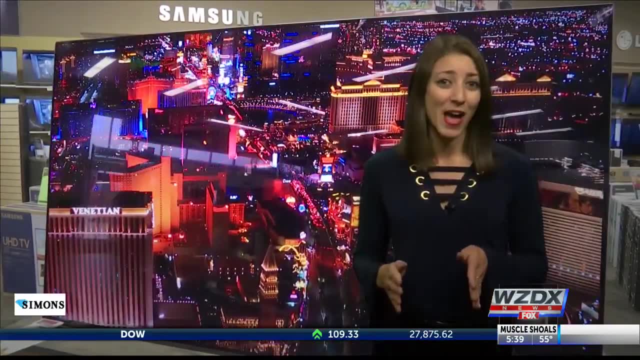 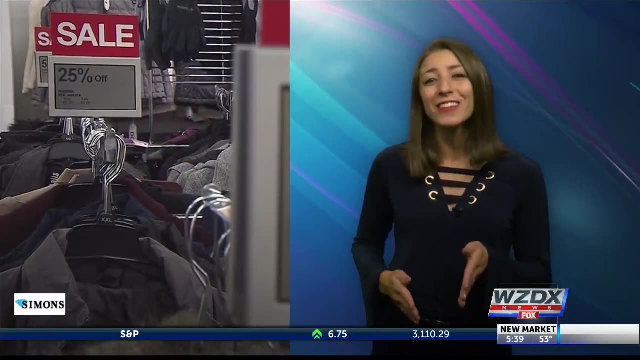 Go online for the best deal on a TV, They say. most online prices are lower, even with shipping. The catch here: Research the company you're buying And read the fine print. Second thing: we're shopping for Clothes. The main consensus on this one: Sales, sales, sales. Keep track of online ones and in-store, because sometimes one is better than the other. 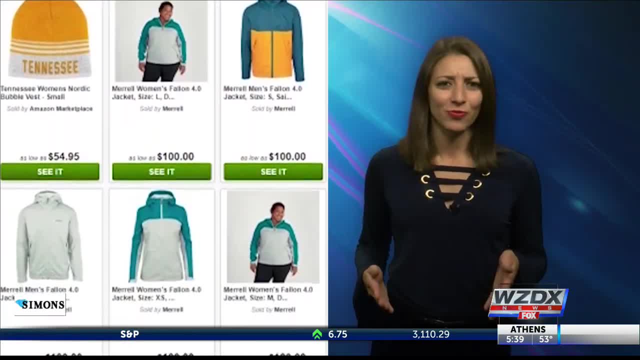 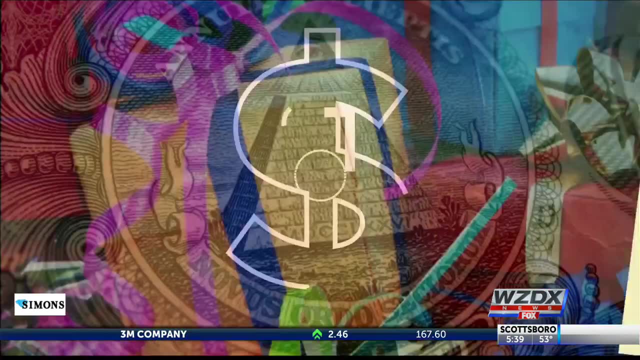 If you're going online, do your research. Are reviews saying the shirt runs big? Is it made out of terrible material? Find out. For some overall tips, we look to consumer expert Clark Howard. First, do your research online to compare prices before going to the store. 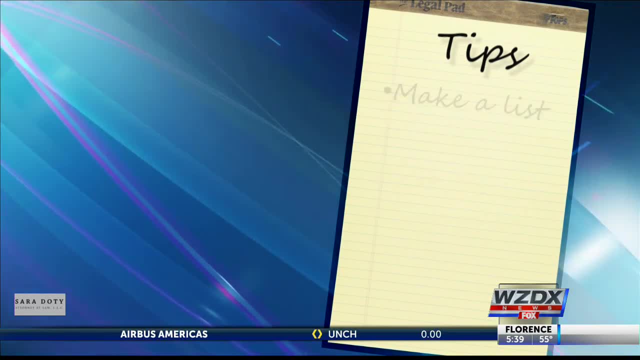 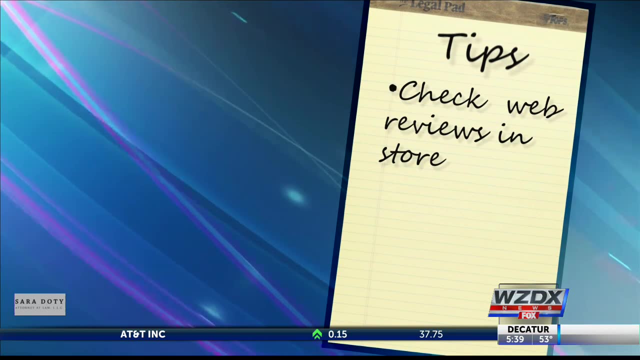 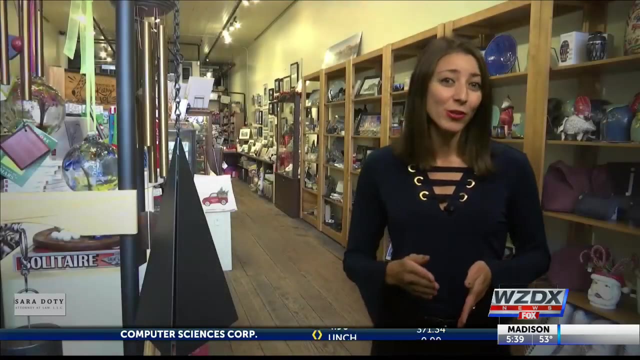 And see if the store will match your prices. Second, make a list and don't impulse buy. Lastly, check out reviews on your smartphone of something you see in the store. So if you're doing all this price comparison, you're probably not doing it at small businesses. Why Where you drop your dollars can matter later in our Smart Shopper series. 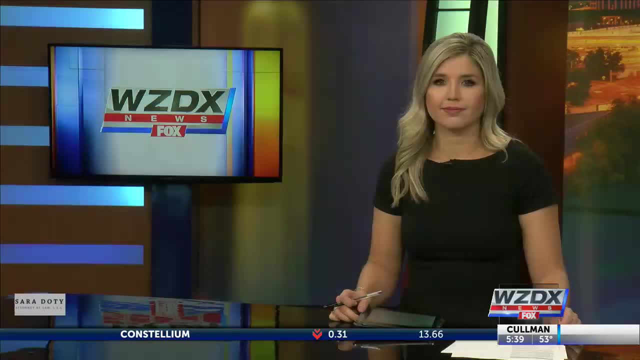 Putting the valley first. Renata DiGregorio, WZDX News. Black Friday means some door busters. you have to go shop in the store for Shop Black Friday to get the newest expensive item. Shop Cyber Monday for older generations of your smaller gadgets.